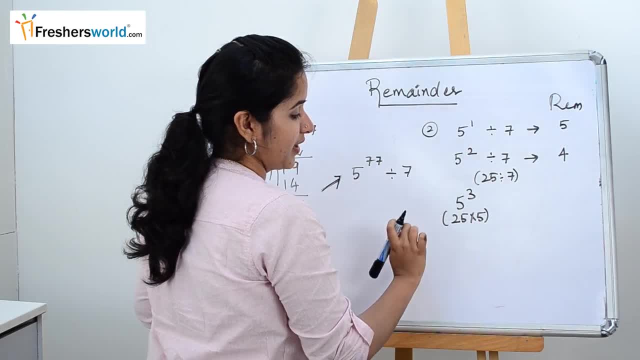 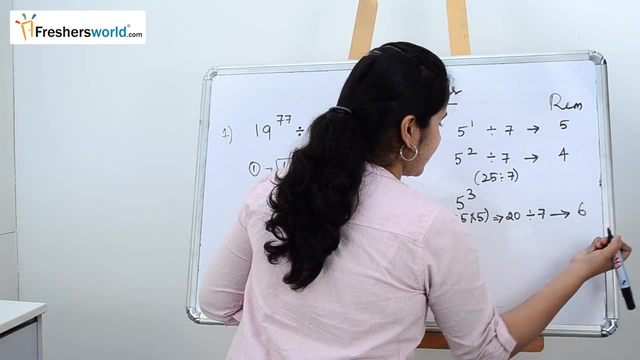 reminder is going to be the same. So 4 into 5, you can do it. This is nothing but 20.. So 20 divided by 7. This is nothing but 6.. So, similarly, next is 5 power 4.. This is nothing. 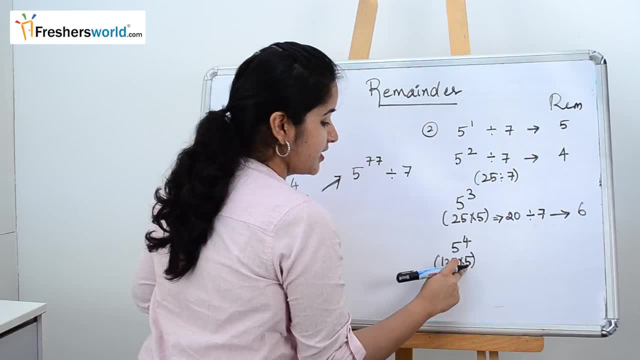 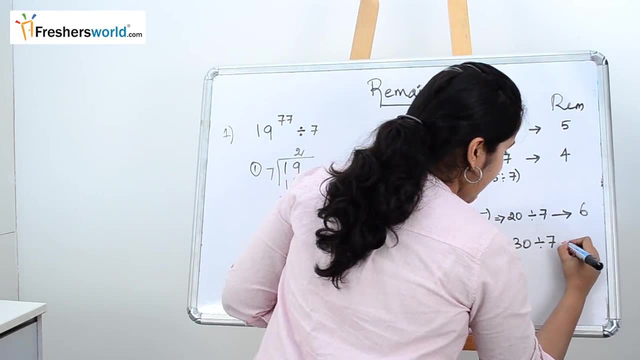 but 125 into 5.. So this is 5 into 6.. This is nothing but 30.. 30 divided by 7.. 7, 4s are 28 and your reminder will be 2.. Similarly, 5 power, 5.. We directly. 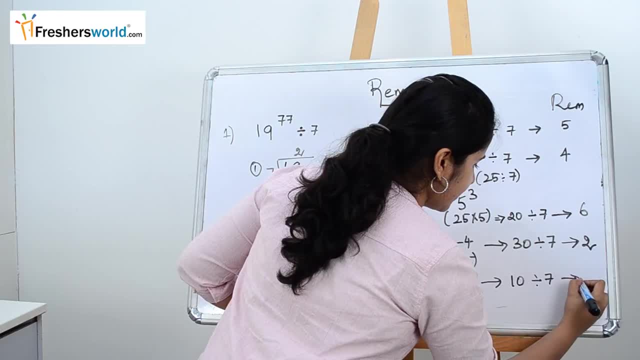 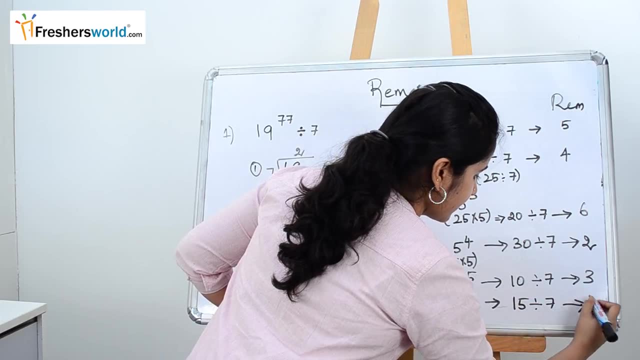 do it now: 5 into 2 is 10.. 10 divided by 7, and the reminder is 3.. And for 5 power 6, it is nothing but 15.. 15 divided by 7 and it's 1.. When it goes to 5 power 7,, now we 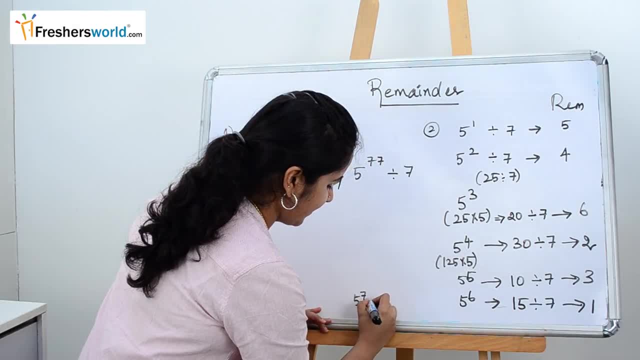 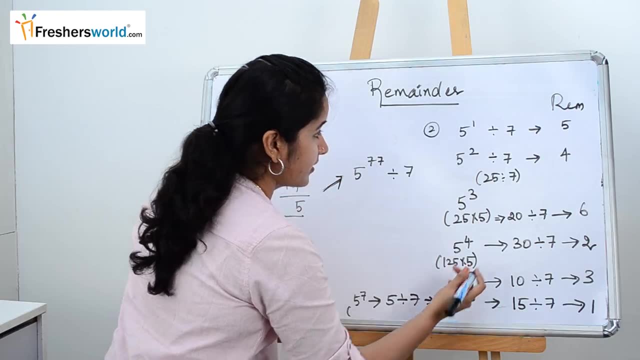 know that we are going to multiply it by 5.. Let's say 5 power 7 is nothing but 15.. We have the reminder 1.. So 1 into 5 is nothing but 5.. It's going to be the same as the first. 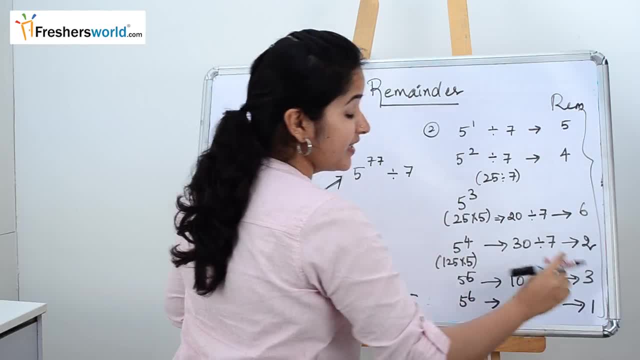 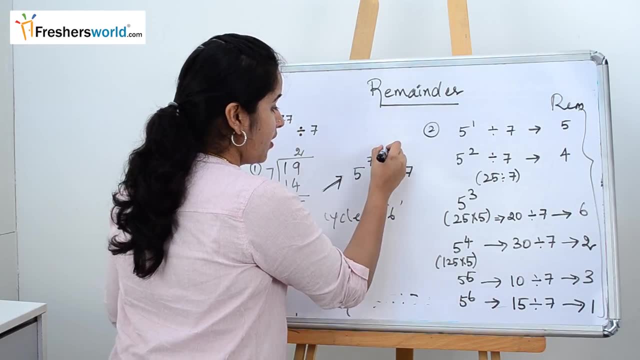 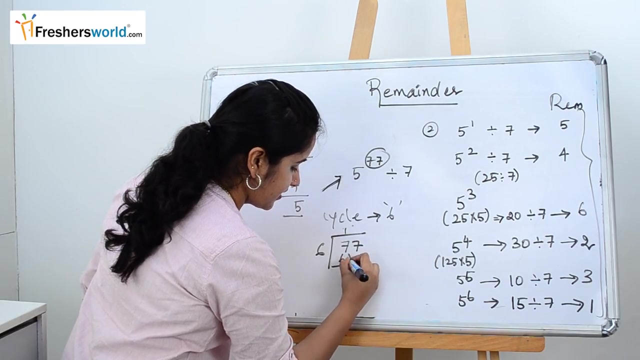 one. So now we understand the cycle repeats every 6 times here. So what do we do it? We know it's the cycle repeats every 6 times. So now take the power. So power is nothing but 77 divided by 6. 6.. We know that 7, 2, 6, 2s are 12.. Reminder is 4.. So this is nothing. 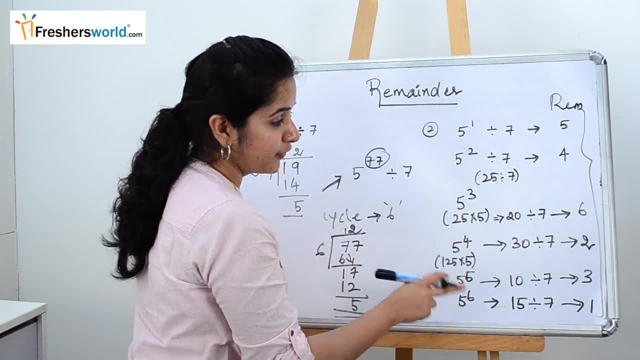 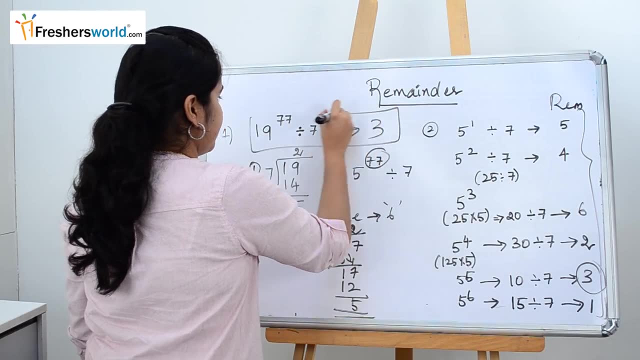 but 7.. Reminder is 5.. So in this cycle, take the 5th term: 1,, 2,, 3,, 4,, 5.. So the reminder of this is nothing but 3.. So how did we do it? Let's have a recap. The first: 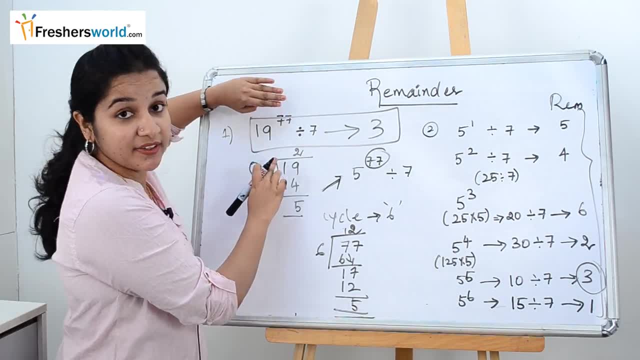 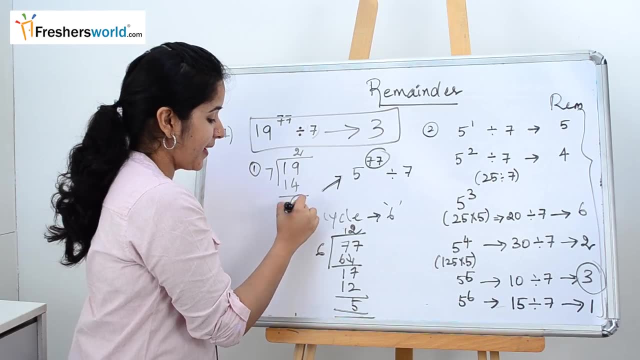 step is that take off the power. Whatever the question that they have given is divided by the value that they have given as a divisor. So 19 divided by 7.. We know the reminder is 5.. So this value, power, 77, divided by 7, is going. 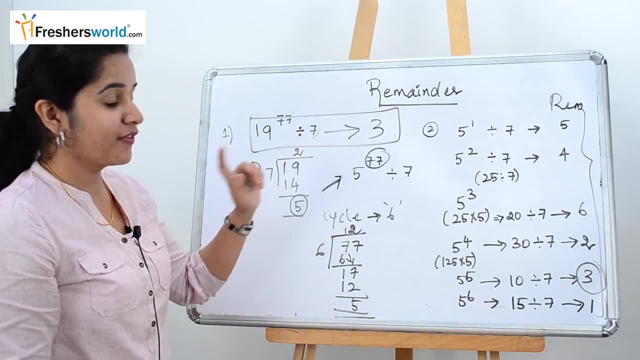 to give you 7.. So this value power 77, divided by 7 is going to give you 7.. So this value power 77, divided by 7 is going to give you the same reminder as the one given in the question. So, first step, we found it out. Now we know to find the cycle of the times.